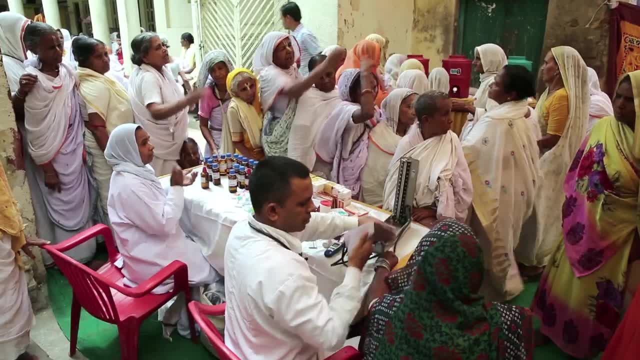 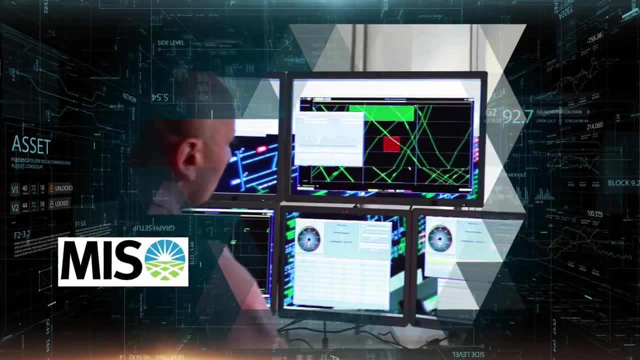 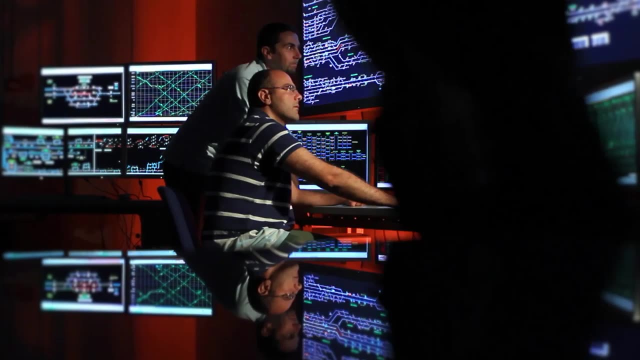 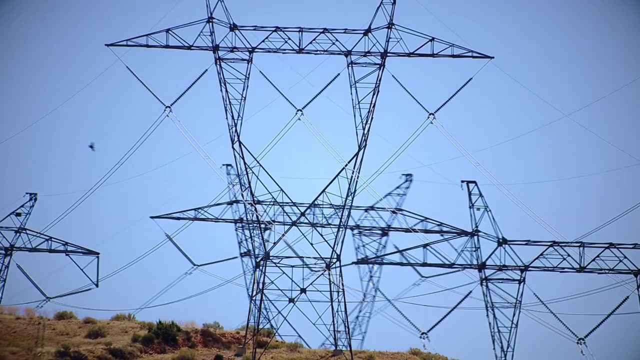 This was wiped out in India, saving countless lives and billions of dollars. MISO leveraged advances in computing capabilities and operations research to launch an energy commodities market that acts as the air traffic controllers of the electrical transmission grid. By notifying power plants every five minutes of the amount of energy required to meet demand, MISO has improved reliability and increased efficiencies of power plants and transmission systems. 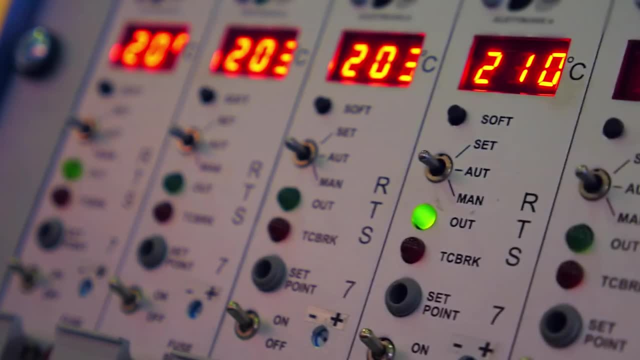 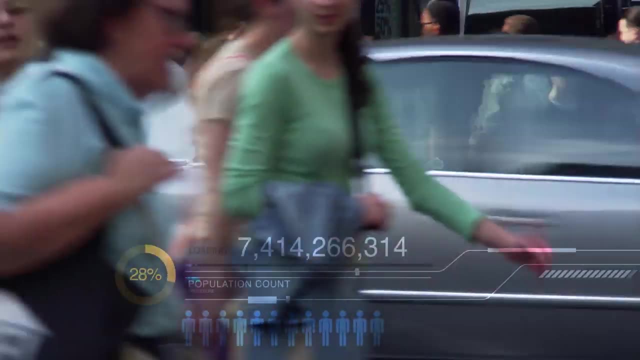 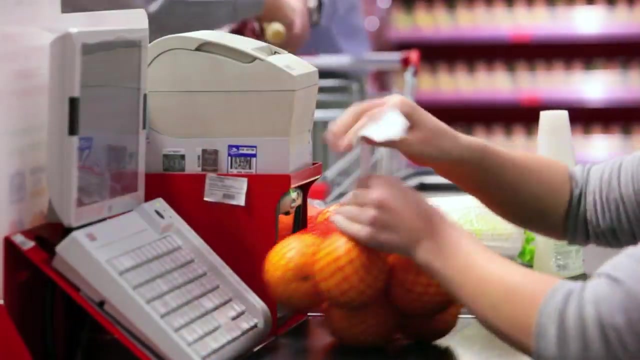 So now there's even more power plants and transmission assets in the Midwest, saving billions of dollars and improving quality of life for millions of residents. With the global population expected to increase by two billion people in the decades ahead, operations, research and analytics are also attacking one of humanity's toughest challenges—producing enough food to feed a fast-growing world. 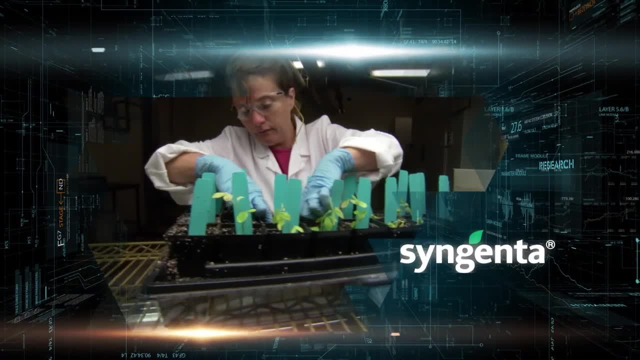 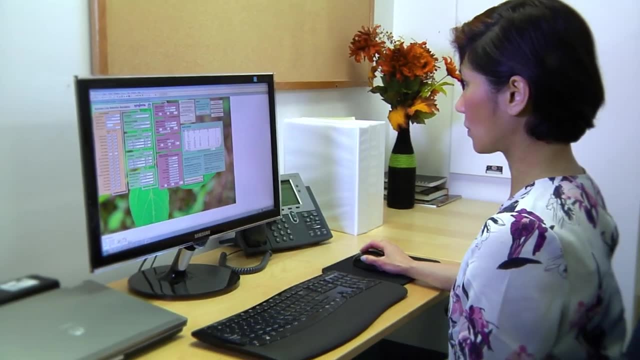 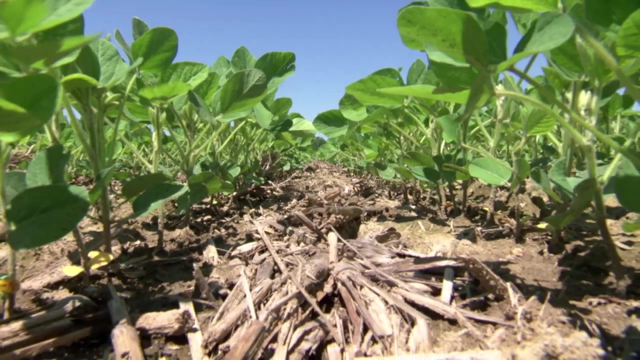 Syngenta's breakthrough approach to addressing this problem was to apply operations research to plant-based agriculture, to plant breeding. By arming scientists with analytics-based decision-making tools, they identified higher yielding crop varieties with a fraction of the effort required under the old-fashioned methods of intuition and guesswork. In 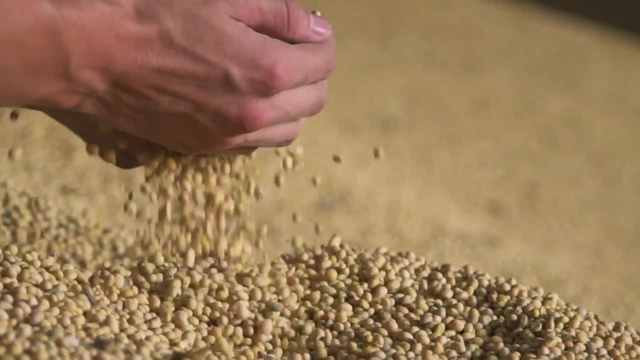 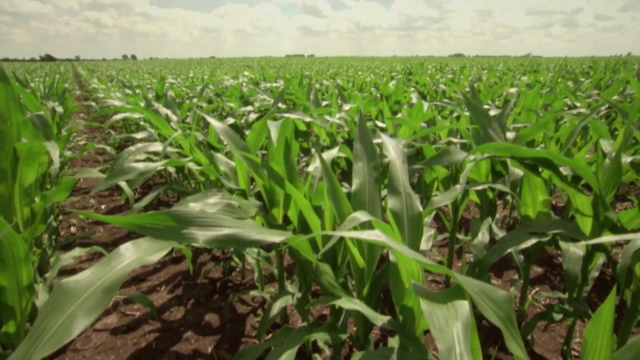 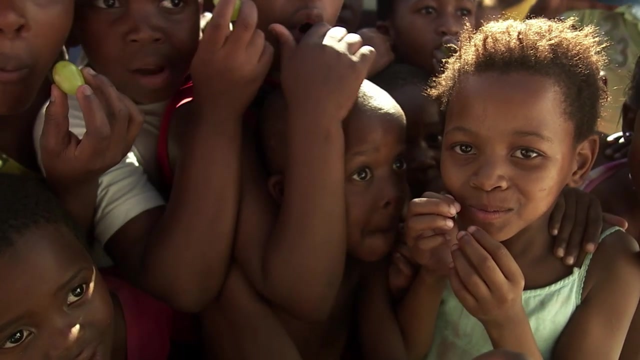 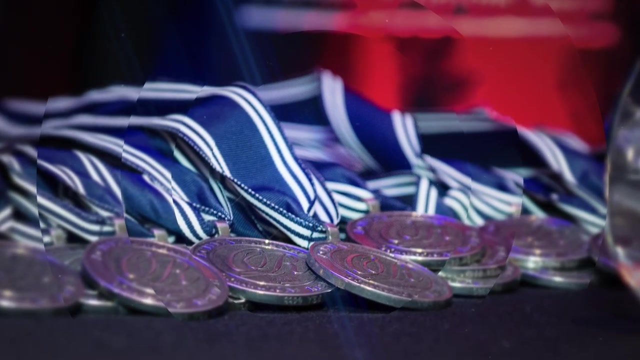 short. Syngenta is using operations, research and analytics to grow more from less, Enhancing farm productivity, helping biodiversity flourish, protecting the environment, improving conditions for farmers and helping to solve the global food security challenge. The Franz Edelman Award is the world's most. 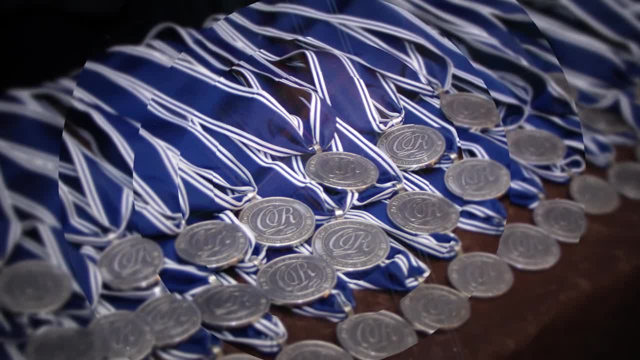 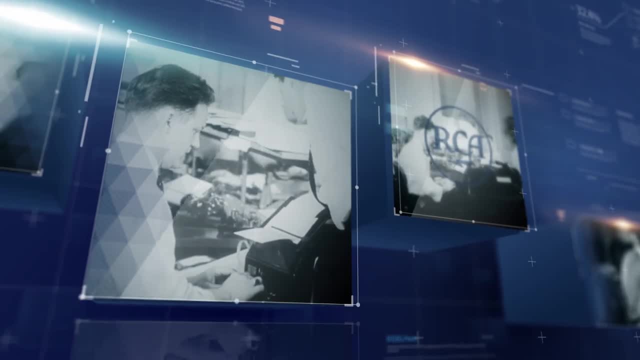 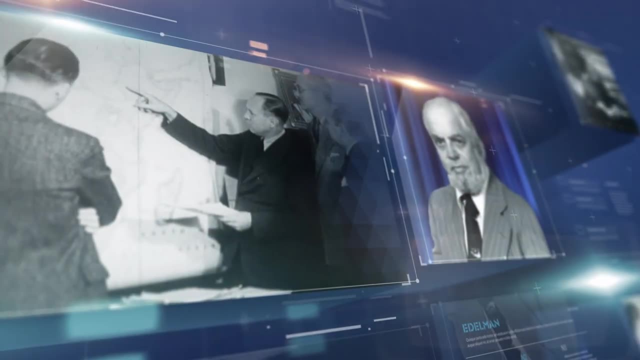 prestigious recognition for achievement in operations research and analytics Named for the man who established one of the earliest operations research groups in the United States at RCA. Franz Edelman is counted among the fathers of innovation in operations research, and he does so because he is an expert in the field of operations research and analytics. 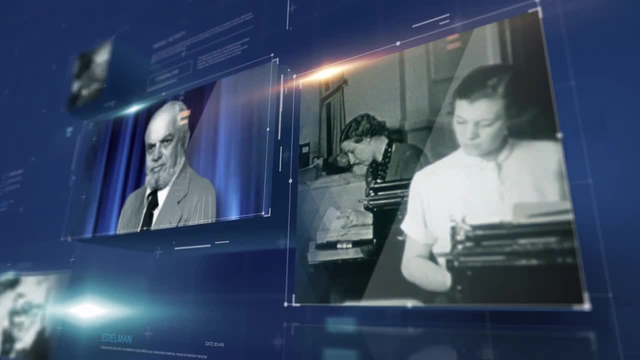 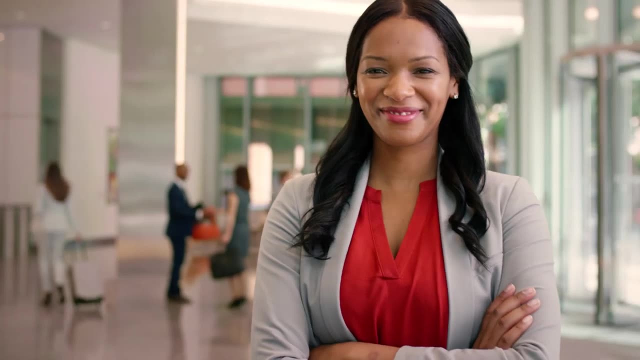 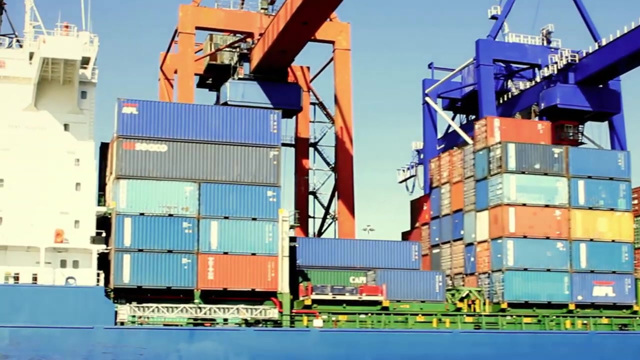 He has dedicated his career to facilitating better decisions on matters great and small through operations research. Today, his discoveries, along with other pioneers in the field, inspire initiatives to help leaders get better results in every sector of management and operations. Every year, operations